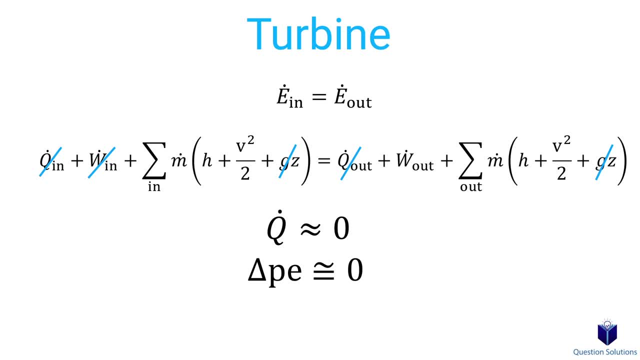 high and these fluids can experience large changes in its kinetic energy. So kinetic energy has to be considered. In certain cases it's possible that this change is relatively small compared to enthalpy change, in which case it can be negligible. So, with all of this in mind, our big energy balance equation for a steady flow system. 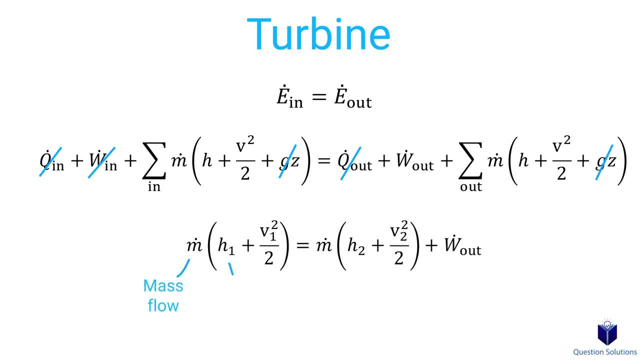 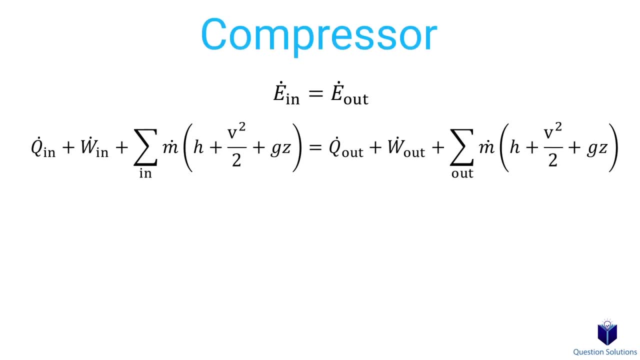 usually simplifies to this. We have mass flow, enthalpy, kinetic energy and, of course, work output. Now for compressors. we already said that it required work input. As with turbines, potential energy is negligible and heat transfer is also negligible unless there's internal. 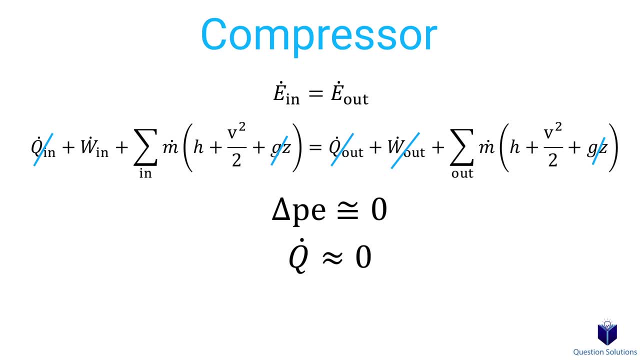 cooling involved. For compressors the velocity change of the fluid isn't significant, so kinetic energy is negligible. So for compressors our energy balance equation is this: In the best case we have an empty equation. usually simplifies to this. We have mass flow work input and enthalpy Notice. 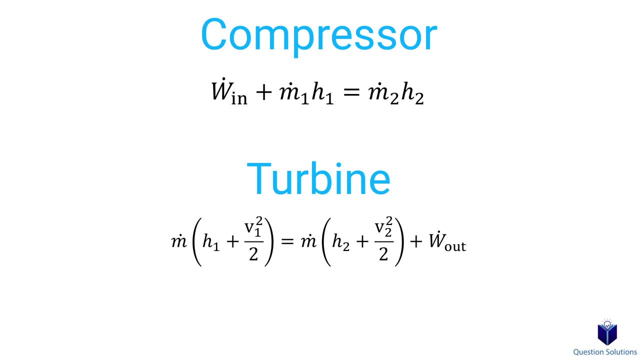 again how for turbines we have work output, while for compressors we have work input. Now let's move on to some examples to see how we can apply what we learned In this question. we have refrigerant 134a entering a compressor and we need to figure. 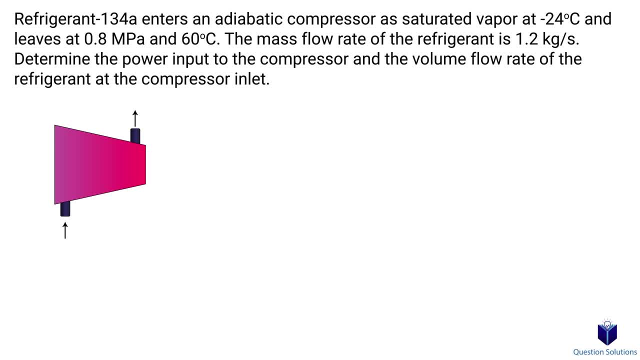 out the power input to the compressor and the volume flow rate of the refrigerant at the compressor inlet. Let's write down what we know. The initial temperature is negative 24 degrees Celsius and final temperature is 60 degrees Celsius. We don't know initial. 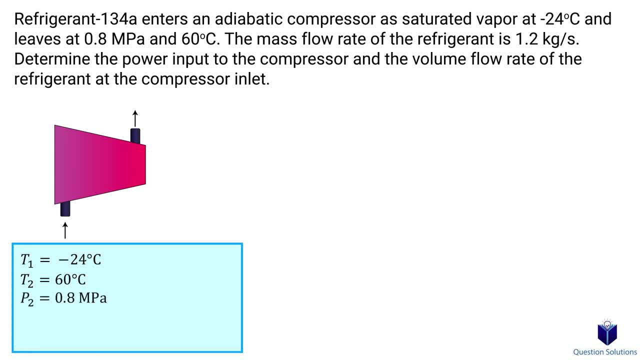 pressure, but we know the final pressure, which is 0.8 MPa. The mass flow rate is 1.2 kg per second. So to find the power input, we can write an energy balance equation. We expand the equation to account for all the types of energy that can be associated with. 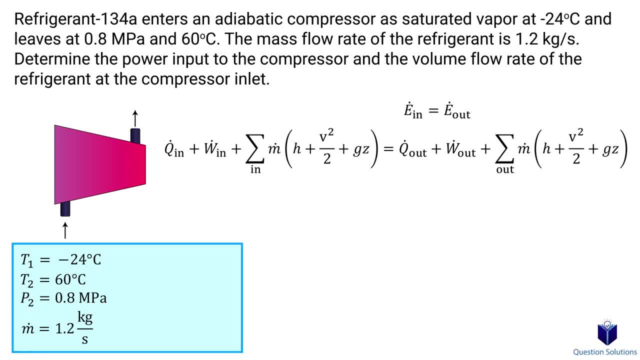 the steady state. Now, since this is a compressor, problem rate of heat transfer, kinetic energy and potential energy is negligible. Again, this is a compressor, which means there is work input but no work output. So our equation simplifies to this. Keep in mind that there is only one input. 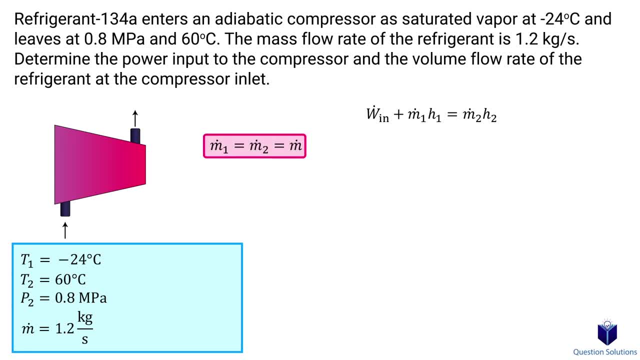 and one exit, which means the mass flow at the input is equal to the one at the exit side. Let's isolate the equation for work input. So, looking at the equation, we have the initial and final enthalpy values. We can find that from the refrigerant table. 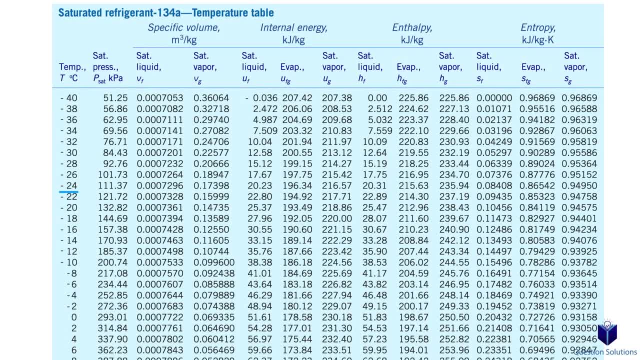 Our initial temperature is negative 24 degrees Celsius and it's the saturated vapor, So our enthalpy value is right here. For the second part of our question, we're going to need the specific volume value And since we have the table up, we can write that down. 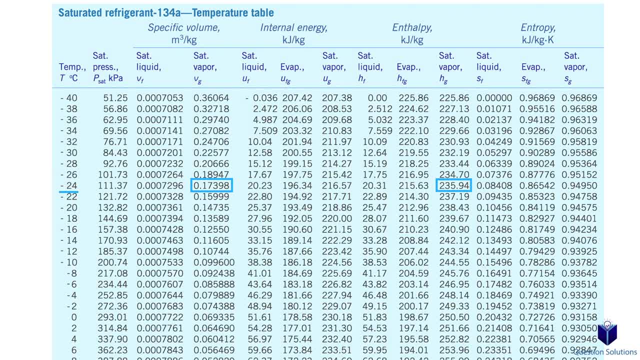 as well. That's the value right here. Next, we need the final enthalpy value. Now it's a superheated vapor and our initial temperature is negative 24 degrees Celsius. We'll write that down as well. Next, we need the final enthalpy value. Now it's a superheated vapor and our 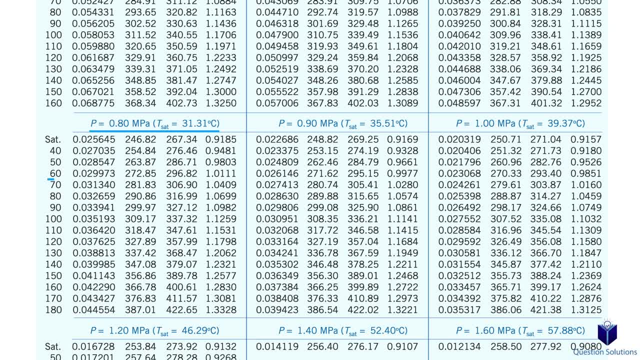 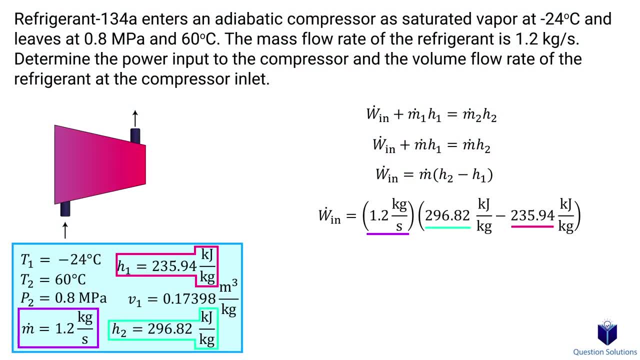 and our pressure is 0.8 MPa and the temperature is 60°C, So our enthalpy value is right here. We can now plug our values in. Solving gives us the power input for this compressor. The next part of the question wants us to find the volume flow rate of the refrigerant. 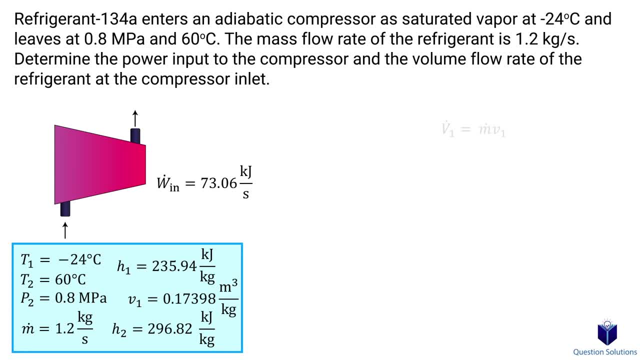 at the inlet of the compressor. For that we can use the equation for volume flow, So that's mass flow times specific volume. We can plug values in straight away, since we already found the specific volume from before. Solving gives us the volume flow at: 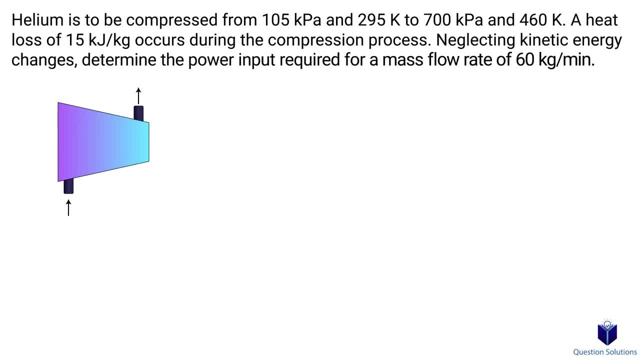 the inlet of the compressor. In this problem, we have helium being compressed and we need to figure out how much power is required for this process. Let's write down what we know. The helium enters the compressor at 105 kPa, with a temperature of 295 Kelvin and a temperature 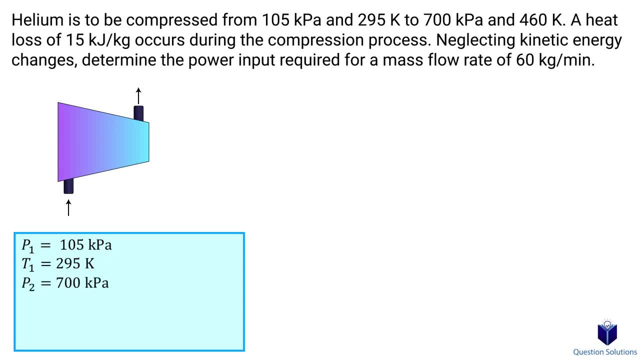 and exits with a pressure of 700 kPa and a temperature of 460 Kelvin. There is a heat loss during this compression process, which is 15 kJ per kilogram and the mass flow rate is 60 kg per minute. We have a slight problem, which is the heat loss and mass flow We need. 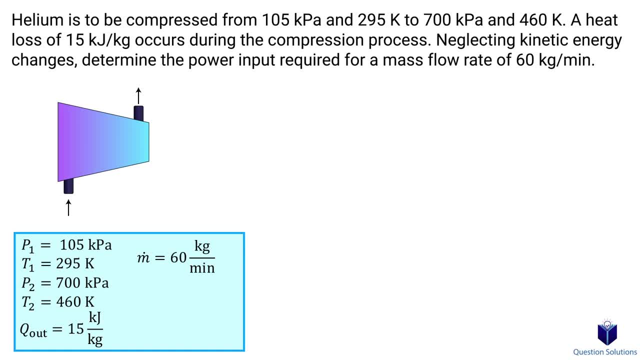 these in terms we can work with. In other words, we need these values to be flow rates that are given with respect to seconds. Mass flow is easy to figure out. We just divide it by 60 and we get this. Now we're told that 15 kJ of energy is lost per every kilogram of helium, And we also 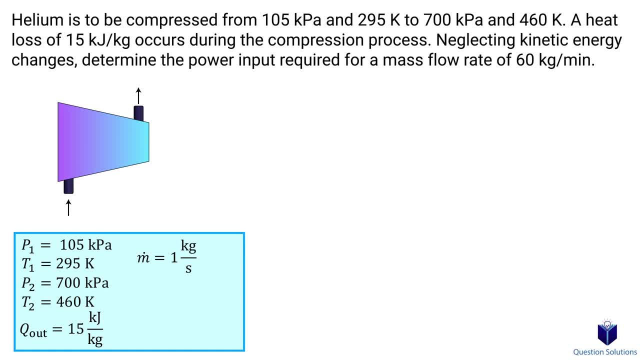 know that 1 kilogram of helium passes through this compressor each second, So that means our heat loss is 15 kJ per second. Now that we have the givens covered, let's write our energy balance equation. This is a compressor problem, so we have power input There is. 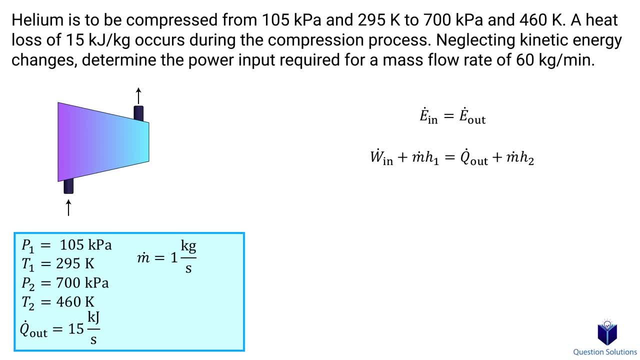 only one inlet and one outlet, so mass flow is the same And we have heat loss. Let's bring the enthalpy terms to one side. We can factor out the mass flow. Now we can find the difference in enthalpy using this equation. All that's left for us to do is 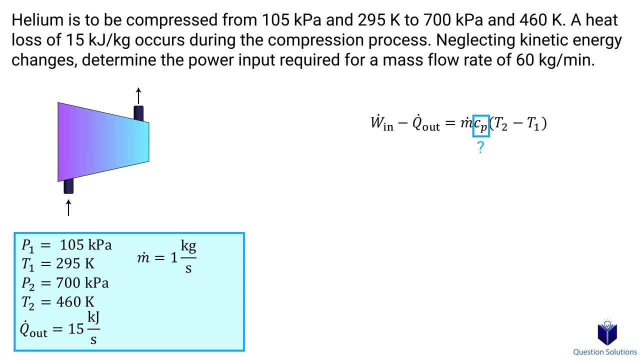 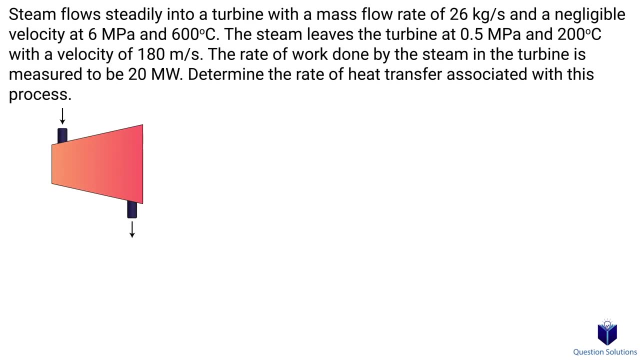 plug values in, but we don't have the specific heat value. So let's look it up on a table for helium. So that's the value right here. Now we can plug our values in. So we need 871.8 kW to run this compressor. In this question we have steam that flows into a 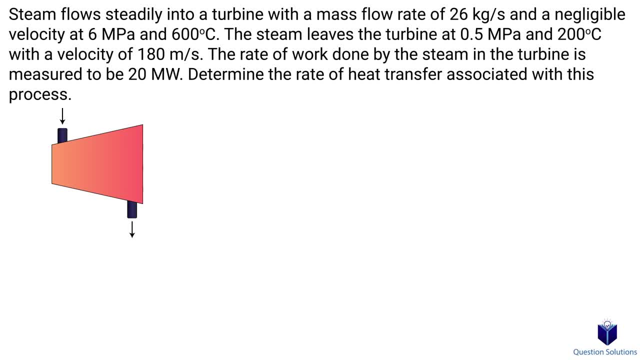 turbine and we need to figure out the heat transfer due to this process. Let's write down what we know. The steam flows in at a rate of 26 kg per second, with a negligible velocity. The initial pressure is 6 MPa and the temperature is 600°C. The steam leaves. 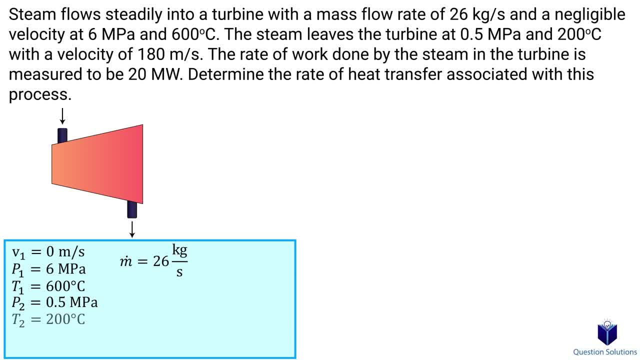 the turbine at 0.5 MPa and a temperature of 200°C, The velocity is now 180 m per second. During this process, the steam produces work which is measured to be 20 MW. Let's write our energy balance equation. 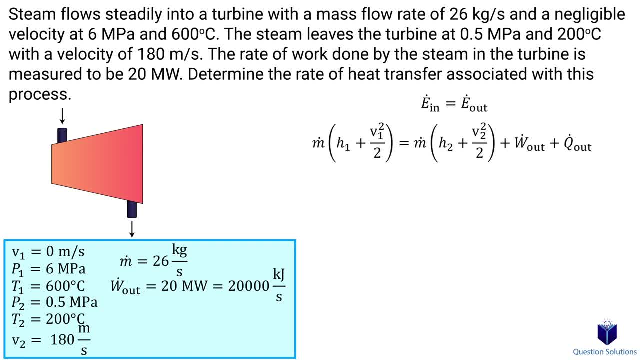 This is a turbine problem, so we have enthalpy, kinetic energy, work output and heat loss. There is no potential energy change. Keep in mind, it's one inlet and one outlet, so mass flow is the same on both sides. So what we need are the enthalpy values, Since 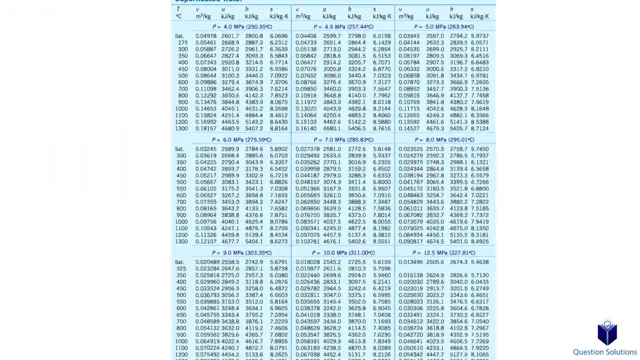 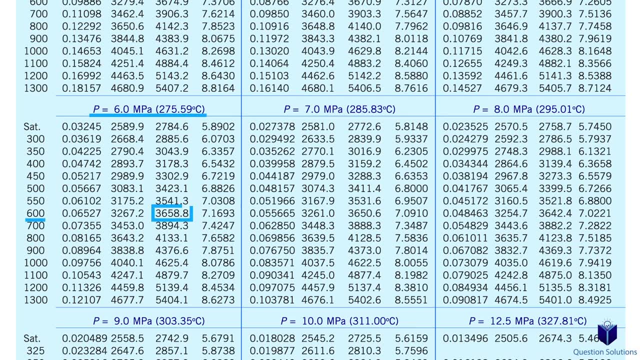 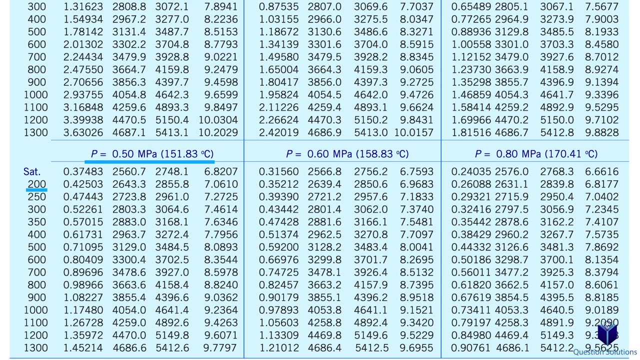 this is steam. we can find those values using a table. The temperature is 600°C, so our value is right here. Our final pressure is 0.5 MPa and the temperature is 200°C, so the value we are looking for is right here. Now we can.